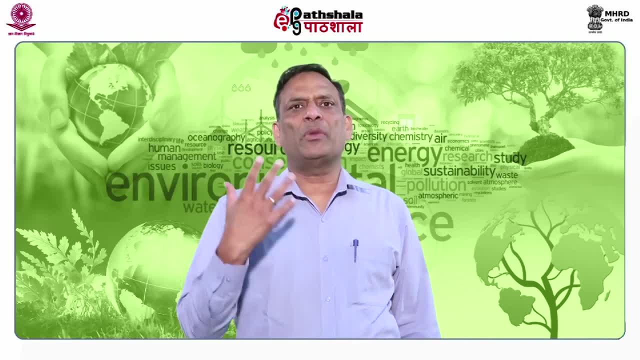 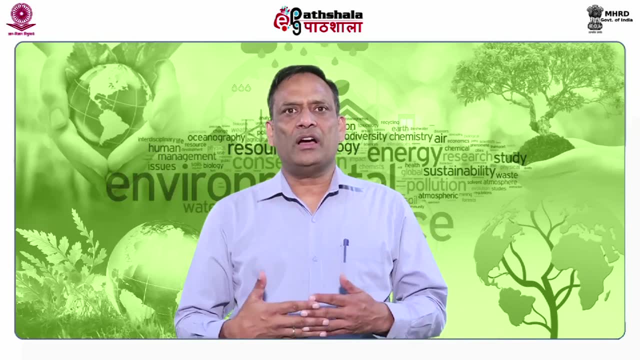 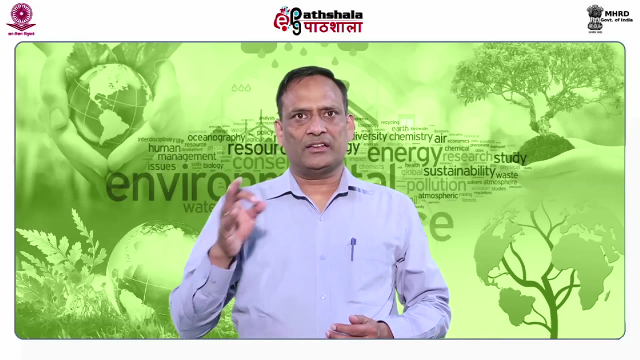 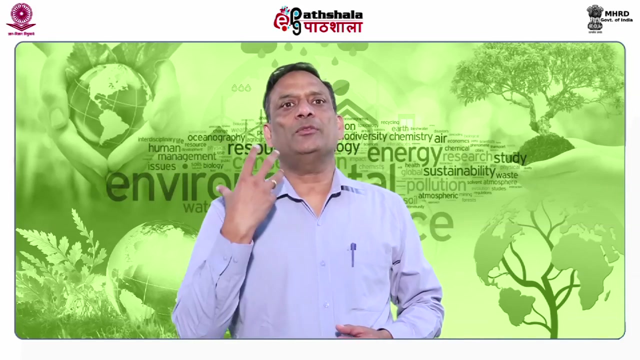 over the globe and what are the mega biodiversity countries, etc. We have also learnt about the applications of biodiversity as well, as we have also learnt that what is the need to conserve biodiversity? So in the biodiversity, we have learnt that biodiversity conservation is very, very important. Now the question arise how it can be conserved. There are a 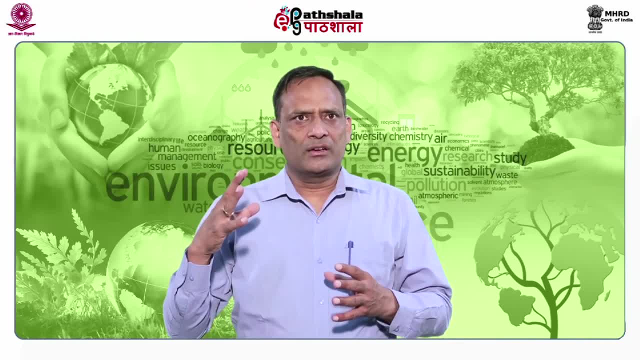 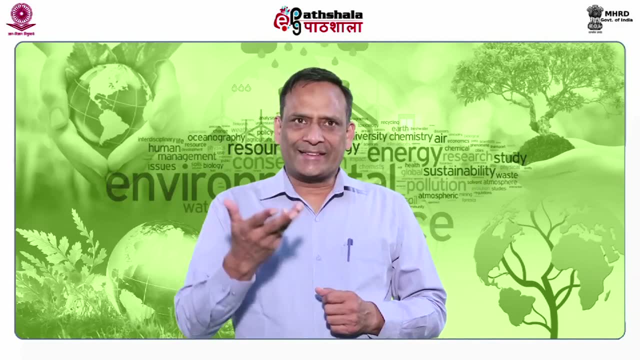 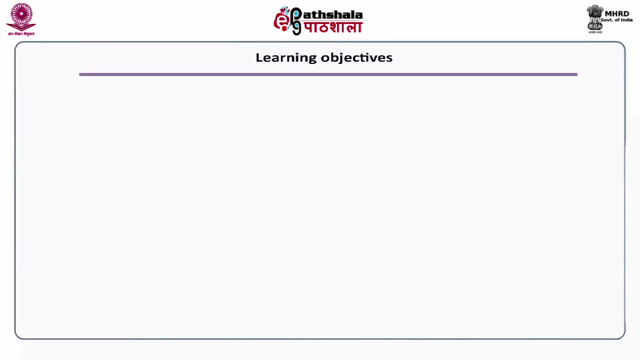 number of ways by which it can be conserved, and one of the way to conserve biodiversity is to use biotechnological tools. that- all biotechnological tools- we will be studying in this module. After studying this module, we will be able to know what are the causes of biodiversity. 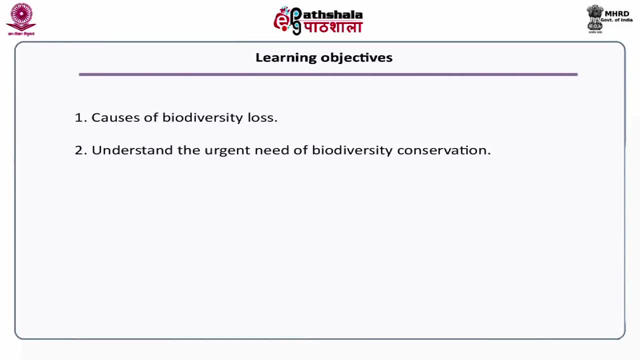 loss, We will understand the need of biodiversity conservation. We will learn about different modes of biodiversity conservation- that is the main theme of this module- and we will also learn about different biotechnological approaches that are available for biodiversity conservation. Now we will try to know about biodiversity conservation. Biodiversity exists in three. 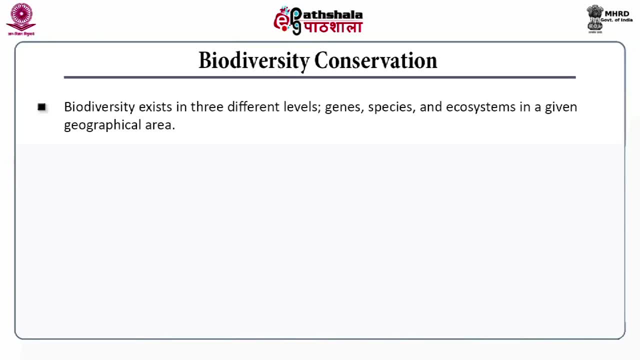 different levels that we have studied earlier. also, just to brief Biodiversity. the three levels of biodiversity are genetic, species and ecosystem biodiversity. in a given geographical area, Each of the component has its own composition, structure and functions in the environment. 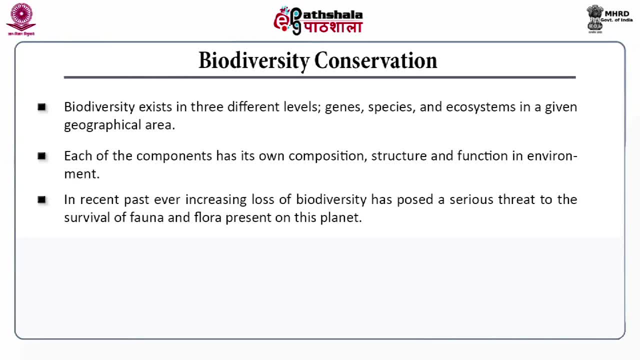 In the late expert, ever increasing laws of biodiversity had posed a serious threat to the survival of fauna and flora present on this planet: Destruction of the habitat of plants and animals, introduction of exotic species- that we will be learning later on in another module- that is, one biological invasion over exploitation of animals and 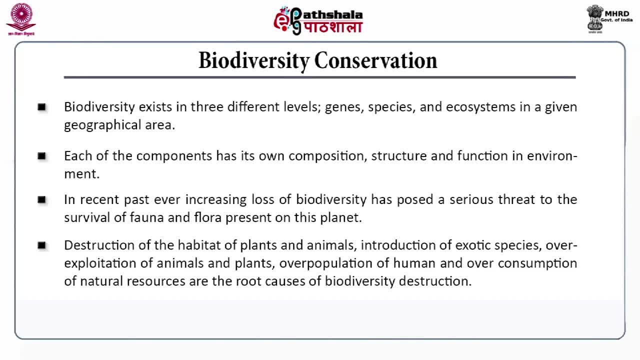 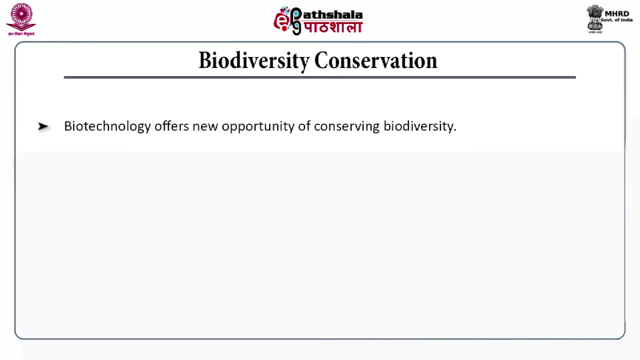 plants to get the goods population of human and over consumption of natural resources are the root cause of biodiversity destruction. So from this all we can conclude, or that there is a urgent need for the conservation of biodiversity As far as biotechnology is concerned. this biotechnology offers several new and innovative. 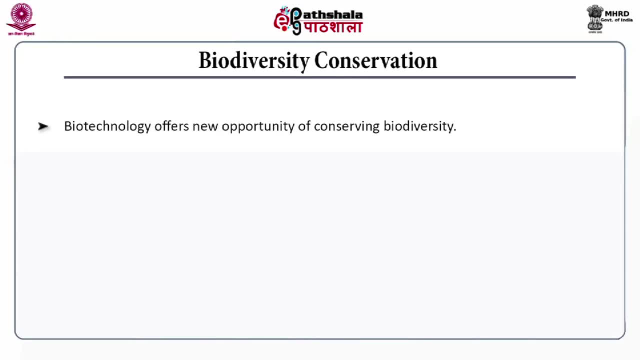 opportunities for the conservation of biodiversity. Now this when we talk about biotechnology. this includes tissue culture, micropropagation, marker assisted breeding, conventional breeding, transgenic crops and genomics. These all are quite beneficial for conserving the biodiversity in several ways. 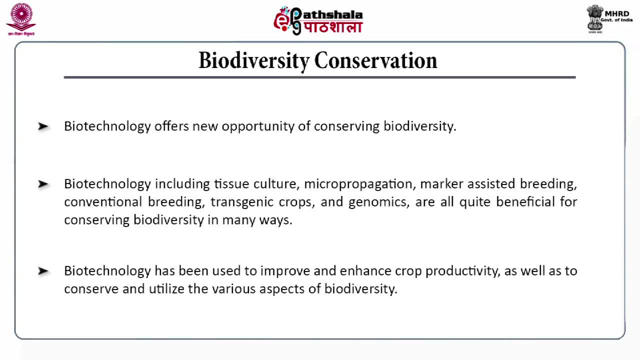 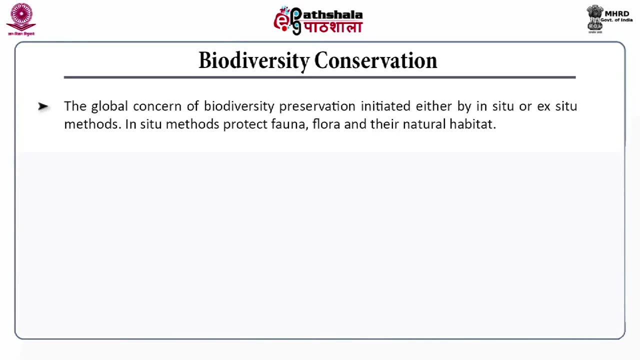 Biotechnology has also been used To improve and enhance crop productivity, that we all know, that the new varieties have been developed, making the use of biotechnology, as well as to conserve and utilize the various aspects of biodiversity. The global concern of biodiversity preservation, initiated either by in-situ or ex-situ methods. 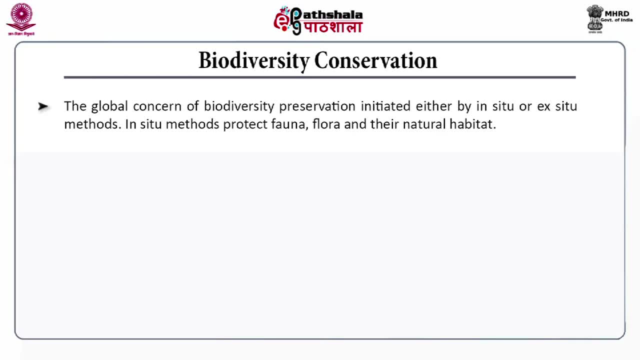 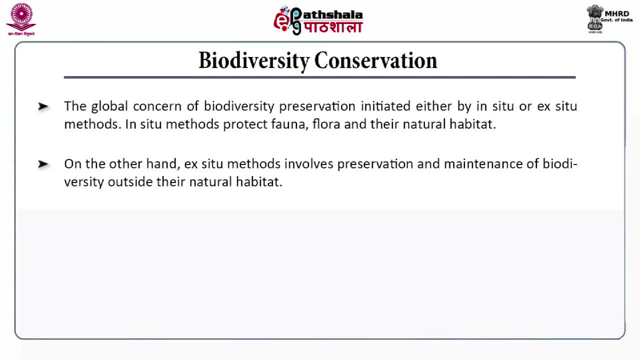 In-situ methods protect flora, fauna and their natural resources. On the other hand, ex-situ methods involve preservation and maintenance of biodiversity outside their natural habitat. Classical methods of plant propagations have certain limitations in terms of rapid production of plant propagules and their long term conservation. 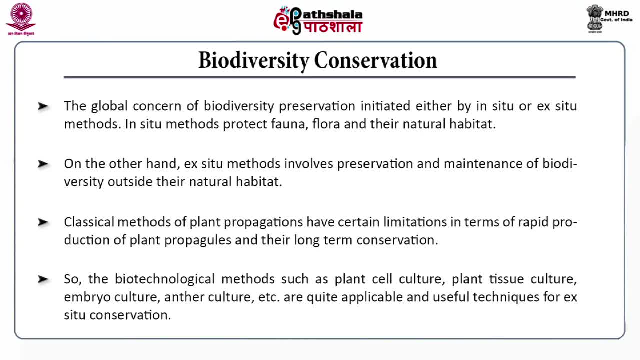 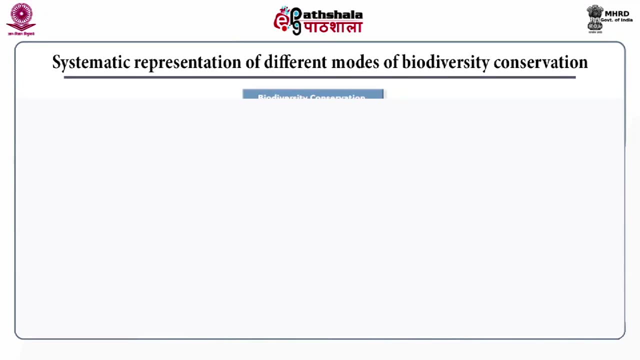 long term conservation. So the biotechnological methods such as plant cell culture, plant tissue culture, embryo culture, enter culture, etcetera, are quite applicable and useful techniques for ex situ conservation. Now, in this figure I have shown about different modes of biodiversity. 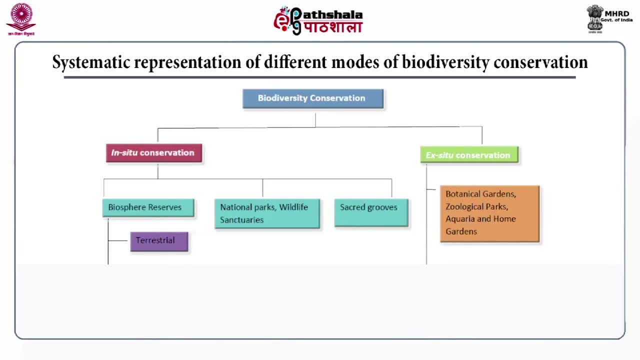 conservation. So one thing we have learnt: there may be two approaches. one is in situ conservation, that is, in the habitat itself, and second one is the ex situ conservation that is out of habitat. So in this figure we will see that what are the different modes? 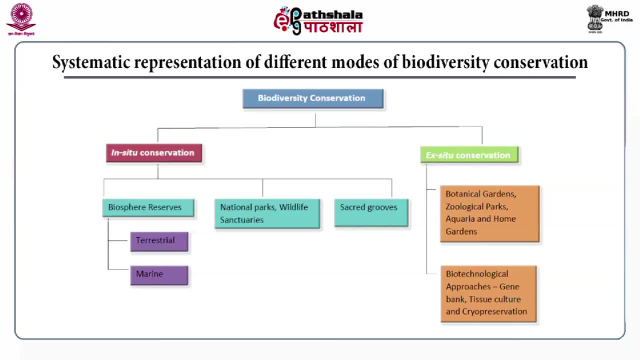 of biodiversity conservation, and these biosphere reserves may be terrestrial, on the land, as well as marine. Then we have national parks, Wildlife centuries- about national parks and wildlife centuries you will be studying in detail in other module. Then sacred grooves. sacred grooves are very old. you can say preservation way of the biodiversity. 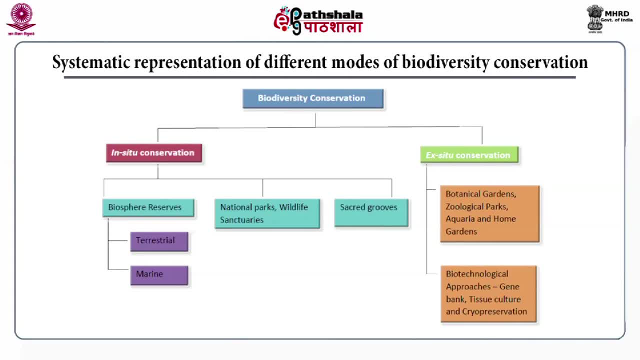 there is not any module on sacred grooves in this paper. I will suggest my students to read about sacred grooves because in recent time lot of attention has been given to the sacred grooves. Sacred grooves as a way of biodiversity conservation and in ex situ conservation. that is another. 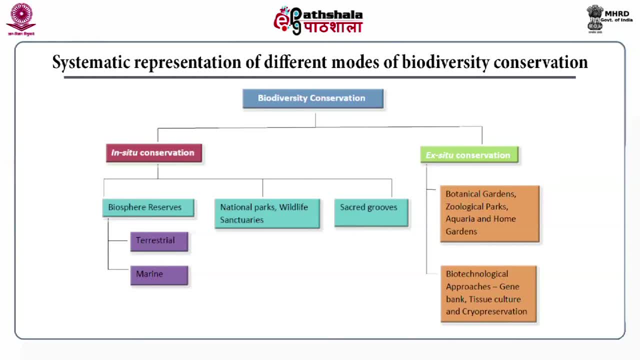 way to conserve biodiversity out of their habitat. We have botanical gardens, geological parks, aquariums and home gardens. In India, home gardens of Kerala are very, very famous. I will suggest the students to learn about the home gardens of Kerala. Thank you. 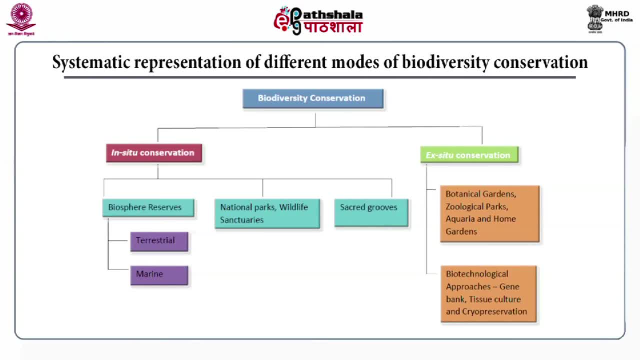 Then comes biotechnological approaches. These biotechnological approaches are ex situ conservation method, and these biotechnological approaches include gene banks, tissue culture and cryopreservation. So these are the different methods, different approaches that can be used for the biodiversity conservation. Now we will be discussing the biotechnological approaches in detail in this. 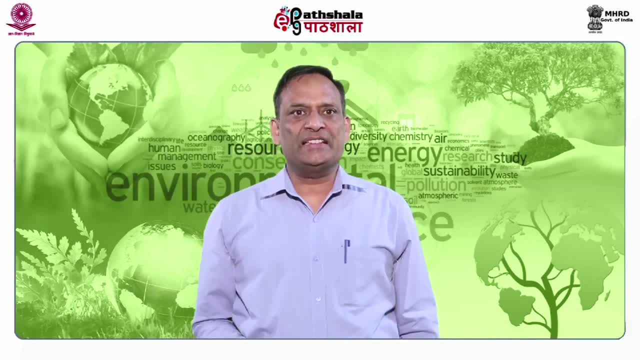 module. Nowadays, loss of specific species- that is called as extinction- or decrease in number of particular organism- that is called as endangerment- are taking place in different of the parts of the world at a rapid rate. Domestic and wild animal species are undergoing a profound erosion process. Conservation of biodiversity through establishment of protected areas like 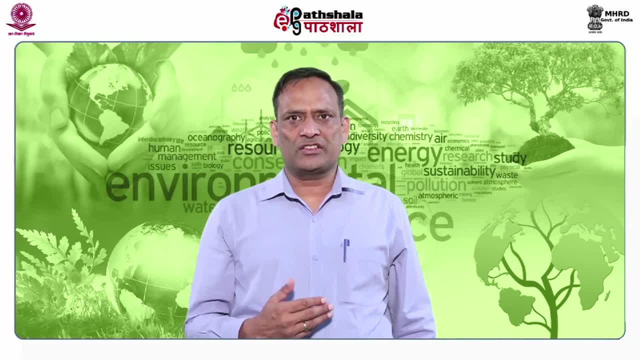 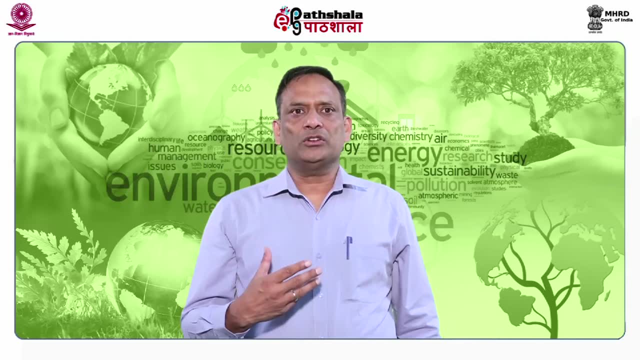 national park, wildlife sanctuary, biosphere and wildlife conservation. These biotechnological approaches that include realities of elevation, polytrophic拿, Walmart, wasteland exhibition, τα- are very effective in controlling the loss of biodiversity. Although biotechnology is commonly 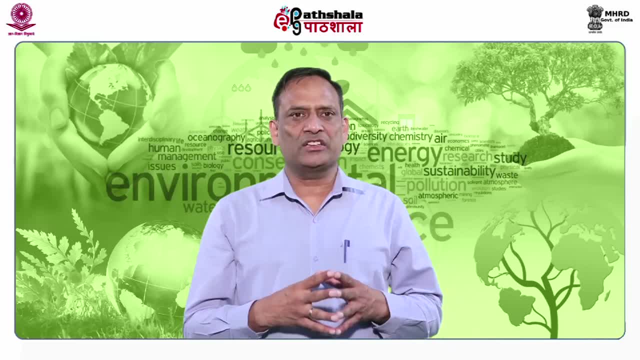 thought of as a recombinant DNA technology. it is used here in a broader term to include tissue culture, cryopreservation, plant micropropagation and animal regeneration from early embryos. Bien гаранкая تهٰ absolutamente 0.. Meeting周خز صند Dh bimientoently. 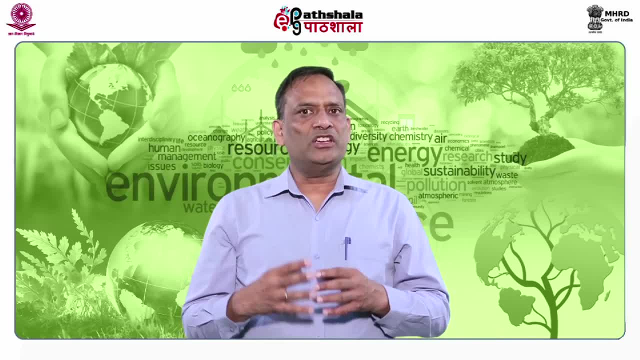 psychological reinforcement of команды phising begonin lateralно ter Φtra and animal regeneration of early embryos. Biotechnology influences germplasm curing, zitten terp symbolise or decomposing the world with diversifying material from the stem cell to. 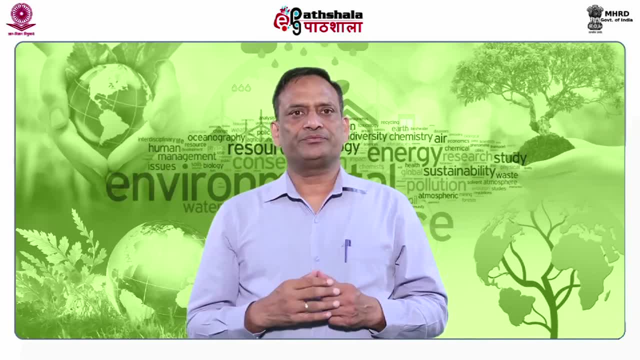 подумan buscando newcomer maker of the 이يін vas 큰 quem beini Bettyą. album of DNA to examine the digestive function of and, by specific evidence, to componに germplasm conservation. in several ways It provides alternatives, in some cases, to conserving whole organism. 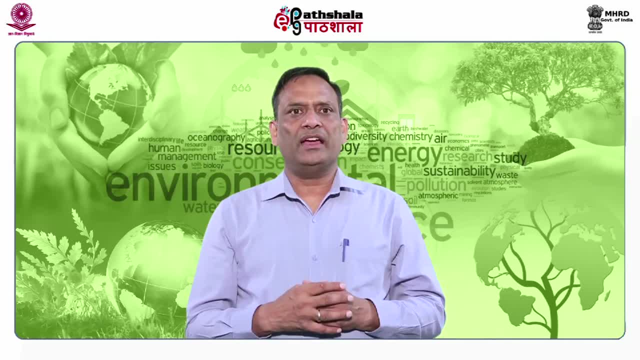 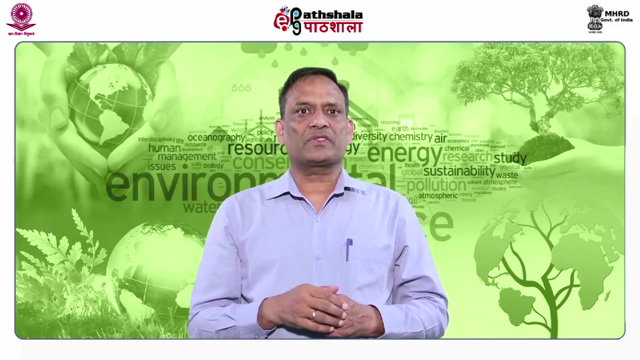 It can assist with the exchange of germplasm, and the techniques of molecular biology can be applied to the problems of managing and using germplasm and influence results from the increased demand for germplasm and conservation services by the biotechnologies themselves. In-situ conservation focuses on preserving the genetic variation in the location it has. 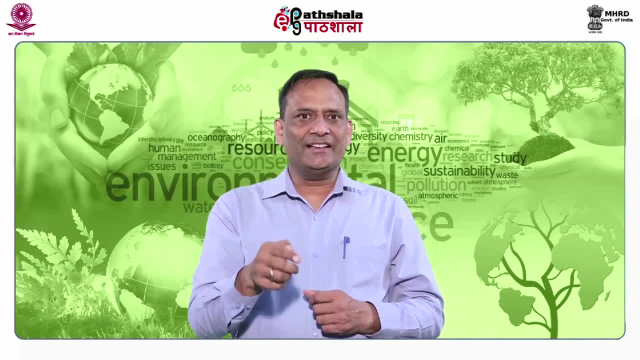 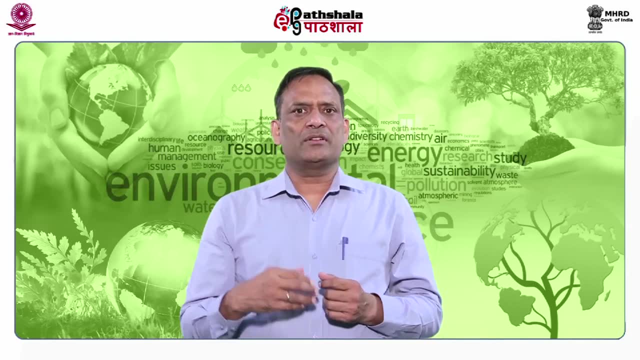 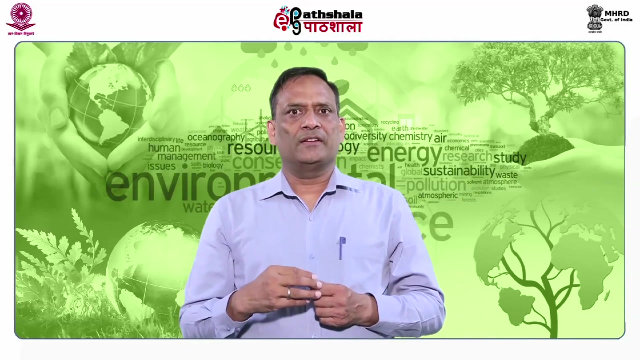 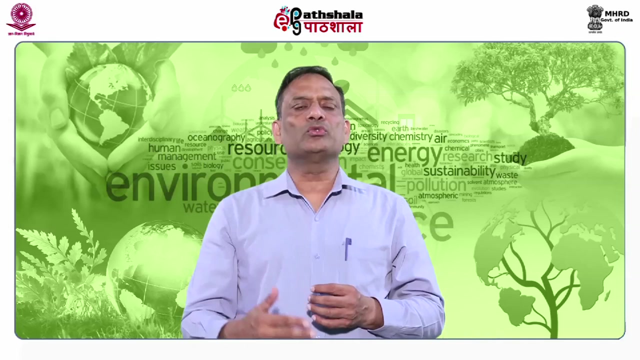 been encountered originally, that is, in its natural habitats, either in the wild or in traditional farming system. In-situ conservation can be carried out At an at any level in any country, without the need for special skills or technology. Properly plant, it can incorporate farmer and industry breeding as well as continued use. 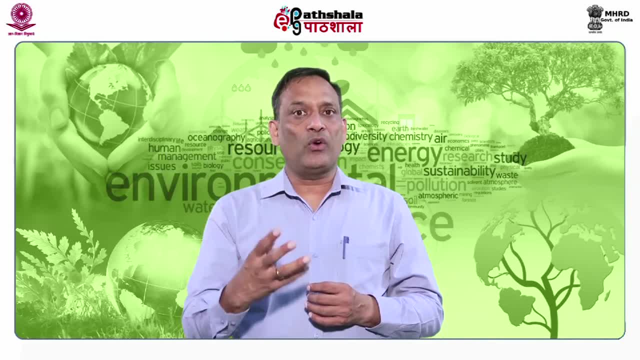 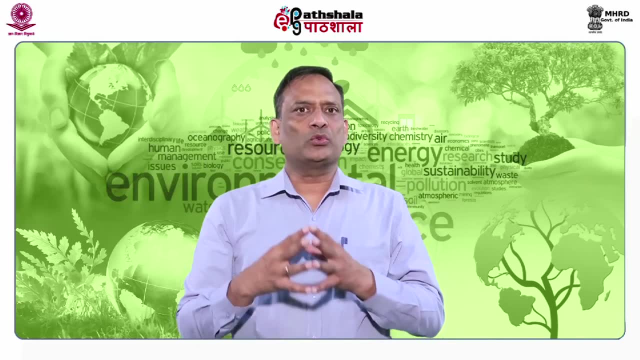 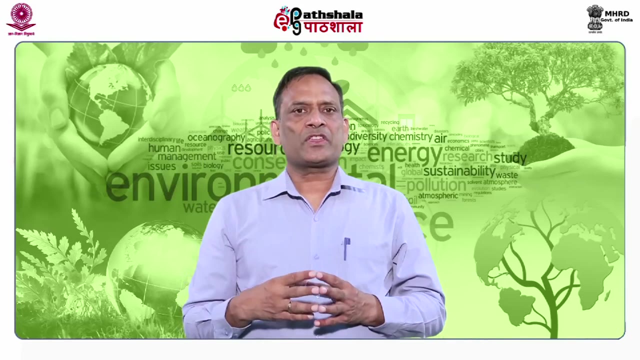 of resources. Now, ex-situ involves conservation outside the native habitat and is generally used to safeguard populations. In-situ conservation includes several methods like seed storage, field gene banks and botanical gardens. Ex-situ conservation of animal genetic resources includes cryogenic preservation techniques. 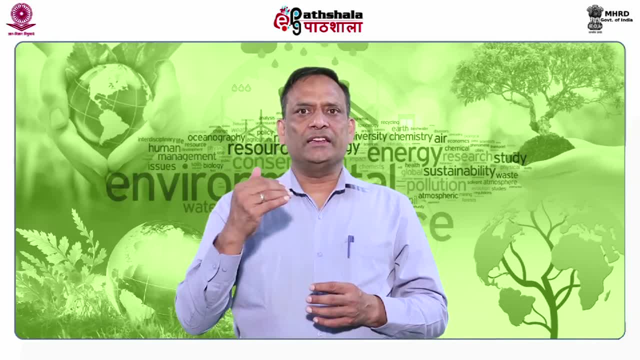 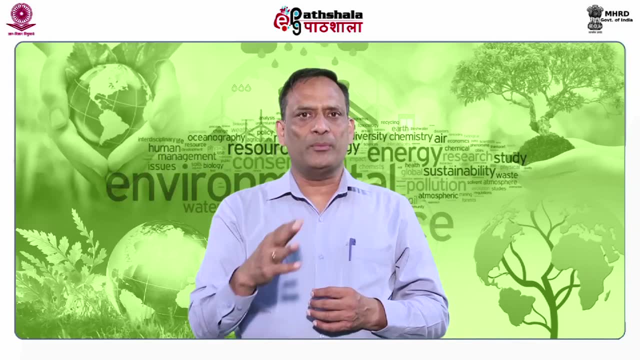 The in cryogenic preservation technique, the collection and freezing in liquid matter of the species or in the soil of the species. In-situ conservation includes several methods like seed storage, field gene banks and botanical gardens, using in liquid nitrogen of semen, ova or embryos or the preservation of DNA segments. 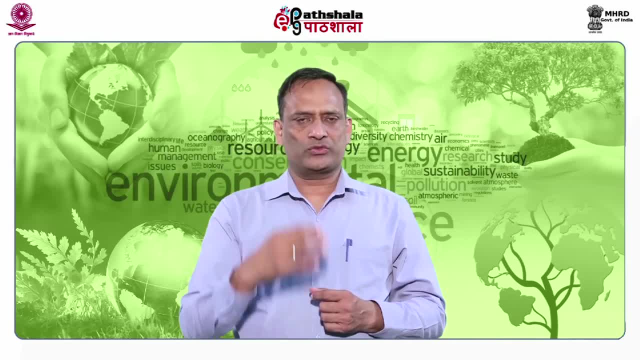 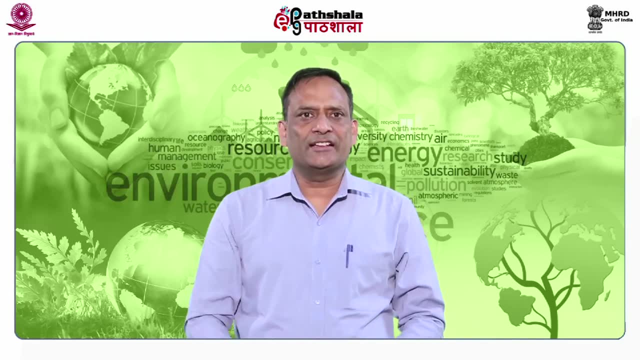 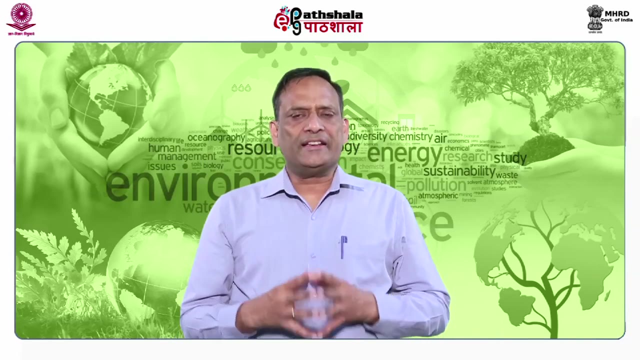 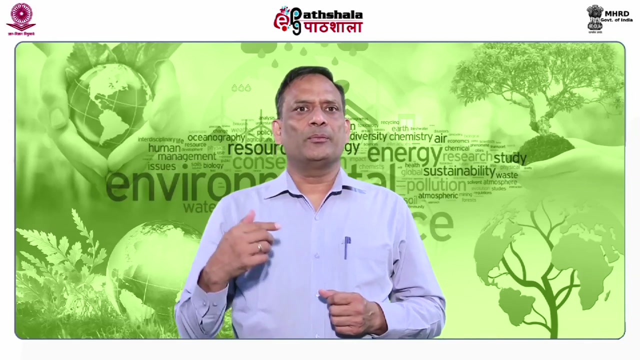 in frozen blood or other tissues. It also encompasses the captive breeding of wild or domesticated species in zoos or other locations away from their natural environment. XC2 gene banks have similar advantages and disadvantages to those used to hold plant germplasm In-situ. 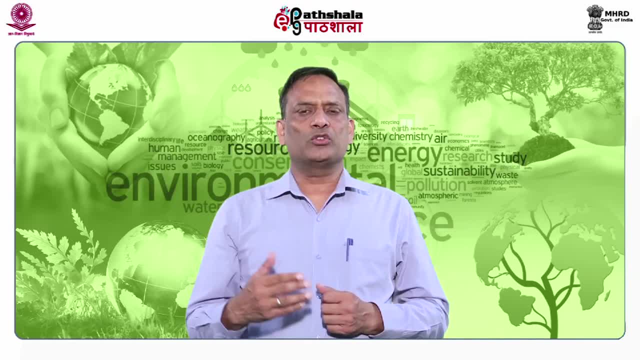 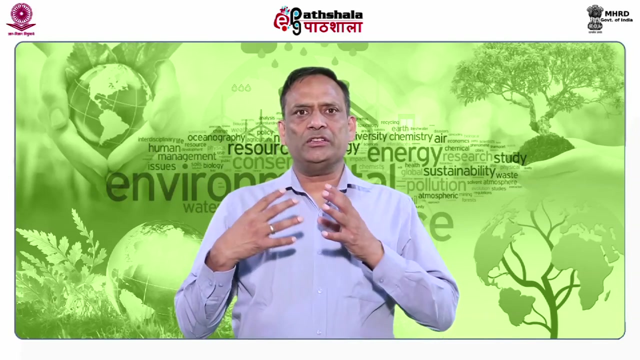 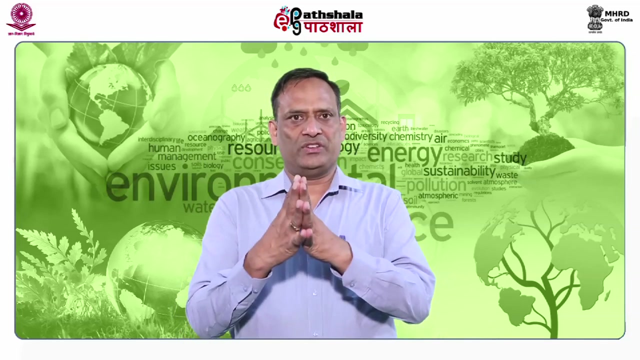 conservation enables animal populations to continue to evolve and be selected for use in their natural environments. It is particularly important for species or within geographical regions where cryogenic problems Preservation is not well developed or available. So the biotechnological approaches of biodiversity conservation come under XC2 mode of conservation. Now, what are different biotechnological approaches? 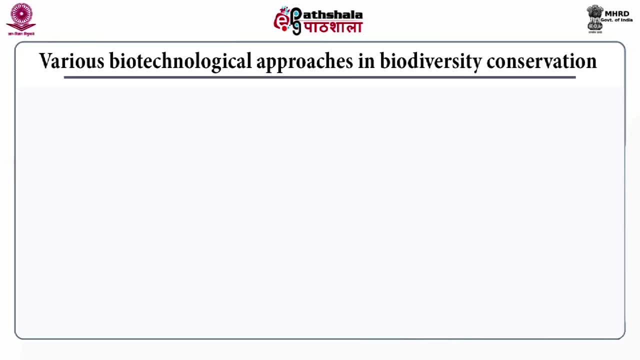 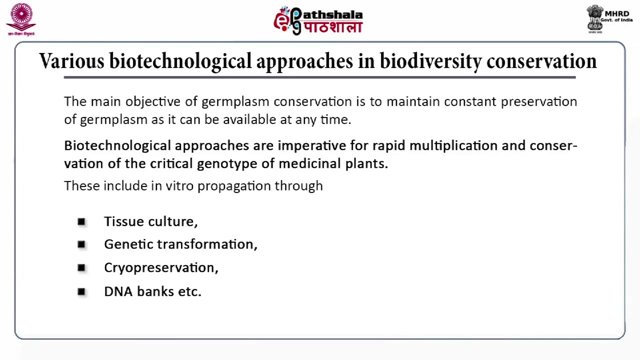 which are used in biodiversity conservation. The main objective of germplasm conservation is to maintain constant preservation of germplasm as it can be available at any time. Biotechnological approaches: Totally Never. propagation through tissue culture, genetic transformation, cryopreservation, DNA banks. 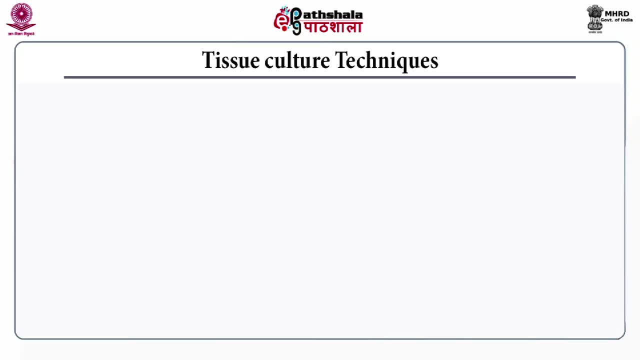 etcetera. Now let me discuss different tissue culture techniques that can be employed for biodiversity conservation. Different tissue cultural techniques that can be employed for this purpose include plant tissue culture, PTC, micropropagation, somatic embryogenesis and organogenesis, and animal. 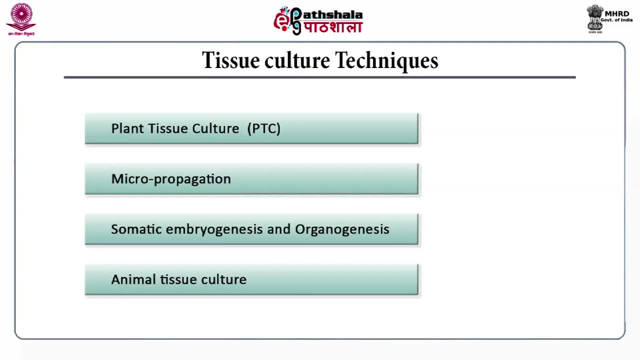 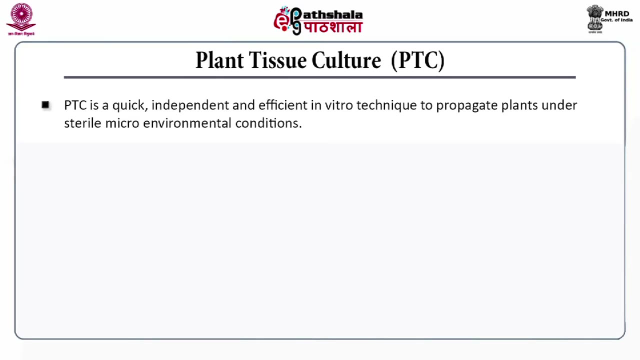 tissue culture. So we will be learning about these techniques in brief. The details of these techniques you will be learning in your paper of environmental biotechnology. Now plant: what is plant tissue culture? Plant tissue culture is a quick, independent and efficient in vitro technique to propagate. 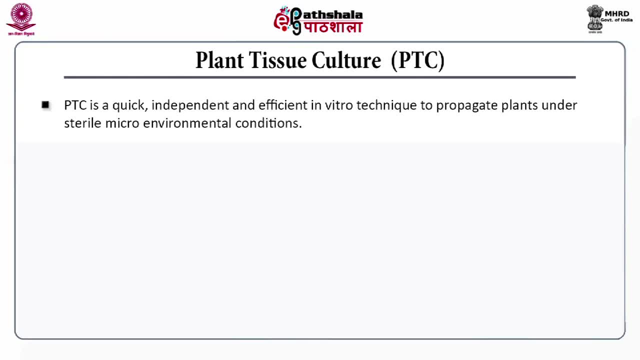 plants under sterile micro environmental conditions. It is very effective method of cloning of plant material and to develop disease free, clean plant stock for propagation. Any plant cell has the power of cellular totipotency. Student should know what is a totipotency, to be differentiated into whole plant in the 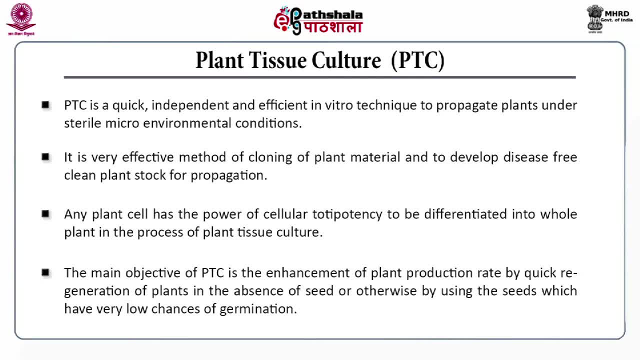 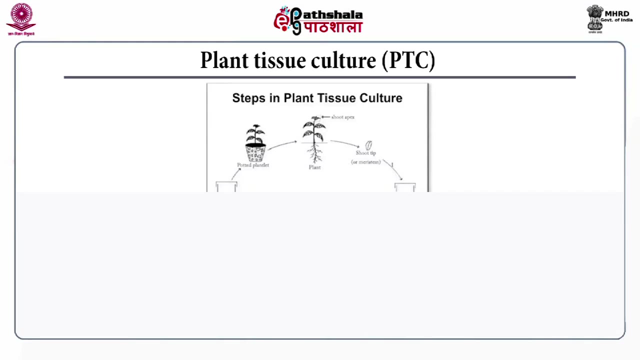 process of plant tissue culture. The main objective of plant tissue culture is the enhancement of plant production rate by quick regeneration of plants in the absence of seed, or otherwise by using the seeds which have very low chances of germination. This figure shows different steps in plant tissue culture. 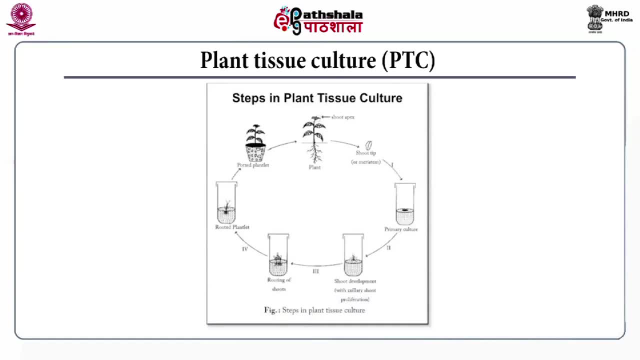 So here, first of all, we have a plant And from the plant We take a shoot tip or meristem. Then this shoot tip is grown in the media or in the culture that is called as primary culture. Student should know that there is not a common media. 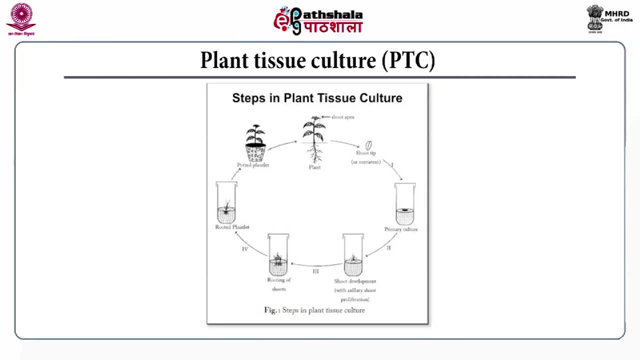 Different type of media can be used for different plants, Then this primary culture in the second step will lead to shoot development. Actually, auxiliary shoot proliferation will take place In the third step. rooting of shoots will be there. In the fourth step we will get rooted plantlets. 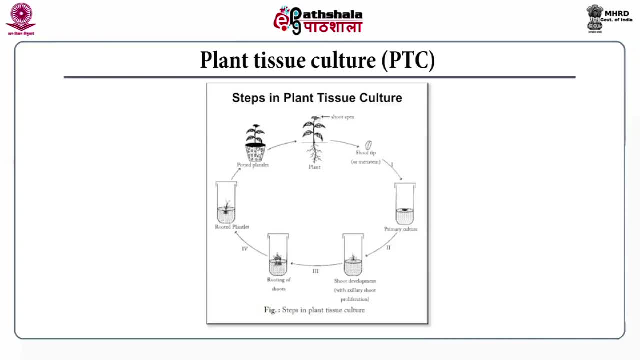 Then these plantlets from the media are potted- called as potted plantlets in the pot, And finally these potted plantlets develop into full plant. So these are the potted plantlets. So these are the total steps, although this process is not that simpler, easy as I have. 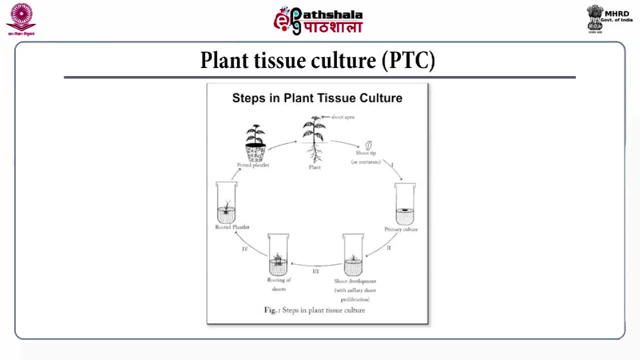 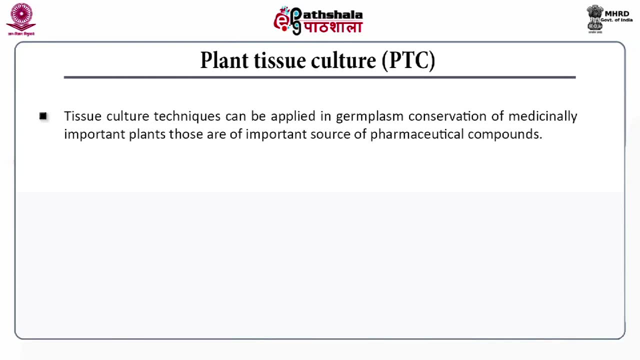 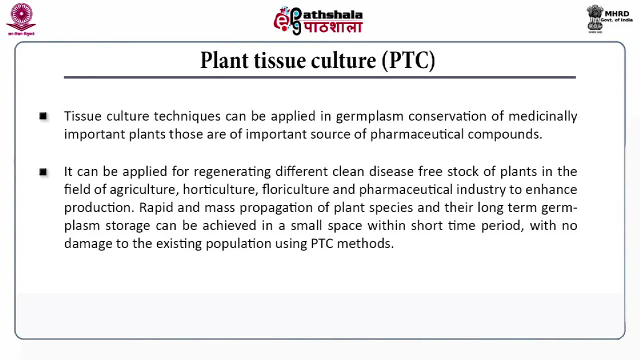 shown here. Process is very complicated and very time consuming. Tissue culture techniques can be applied in germ plasm, conservation of medicinally important plants, important source of pharmaceutical compounds. It can be applied for regenerating different agrochemical. Indonesian therm 불리В. 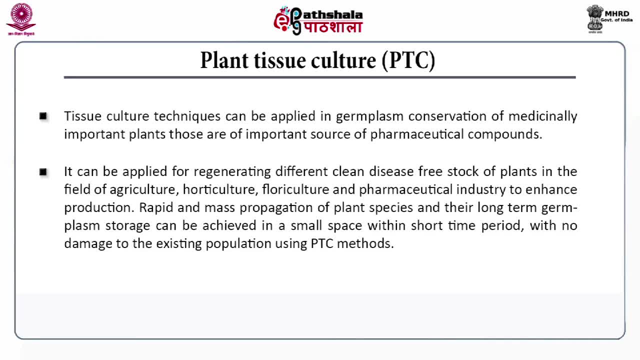 of plants in the field of agriculture, horticulture, floriculture and pharmaceutical industry to enhance production. Rapid and mass propagation of plant species and their long-term germplasm storage can be achieved in a small space within short time period, with no damage to the existing. 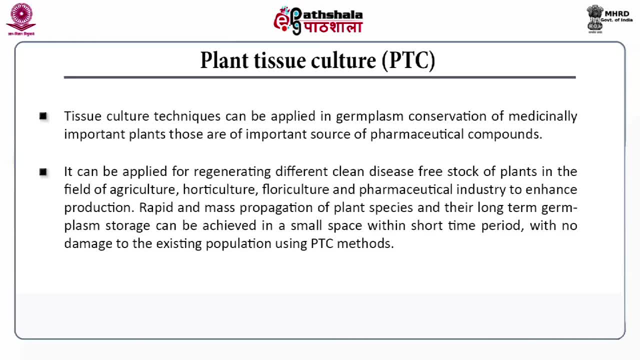 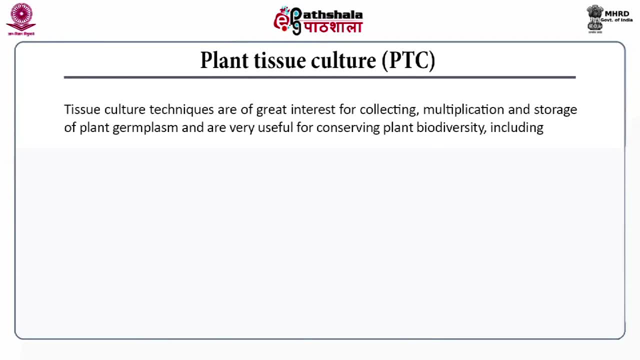 population using plant tissue culture methods. Tissue culture techniques are of great interest for collecting, multiplication and storage of plant germplasm and are very useful for conserving plant biodiversity, including genetic resources of recalcitrant seed and vegetatively propagated species. Rare and 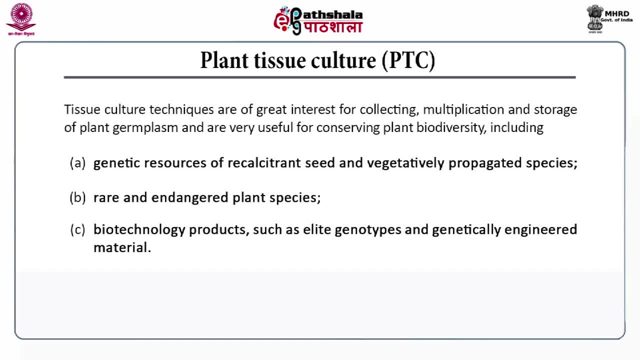 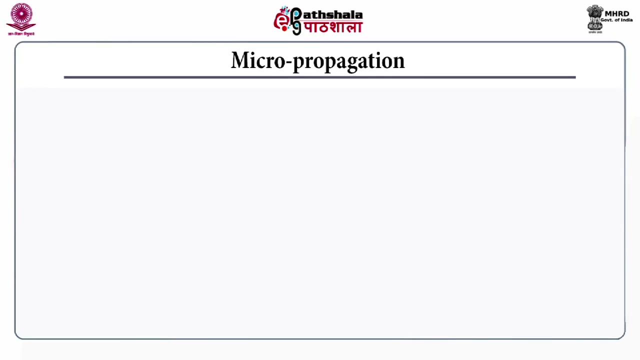 endangered plant species and biotechnology products such as elite genotypes and genetically engineered materials. Tissue culture systems allow propagating plant material with high multiplication rates in an aseptic environment. The second technique that can be used for biotechnological this biodevastation. 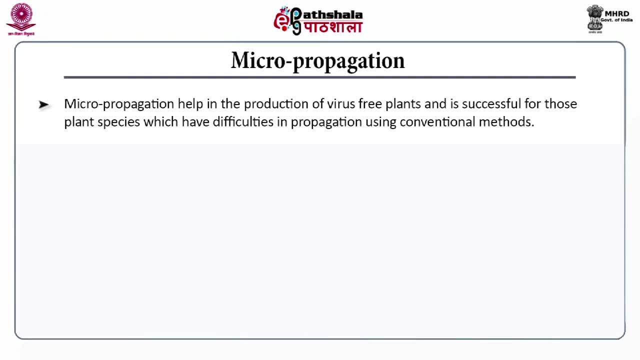 conservation is micro propagation. Micro propagation helps in the production of virus free plants and is successful for those plant species which have difficulties in propagation using conventional method. It is an in-situ conservation of plant species having special phenotypic characters by introduction of regenerated plantlets. 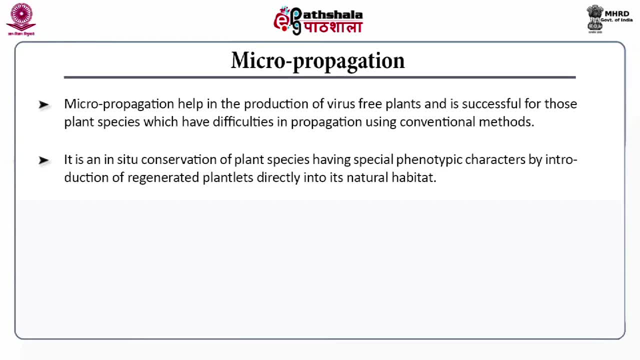 regenerated plantlets directly into its natural habitat. In a short period of time and limited space, it allows the production of numerous plant species. The selection of the explants is very important for the successful micro propagation which decides the final fate of the developed plantlets, via callus or without formation of callus. 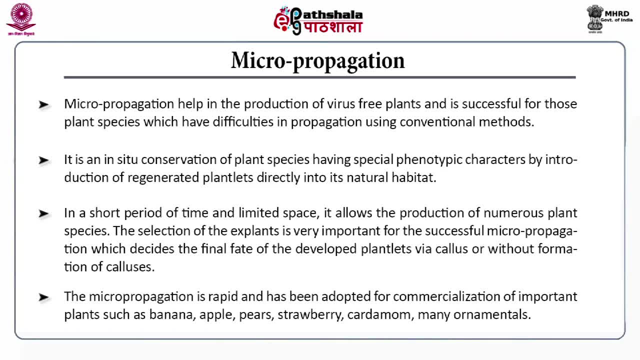 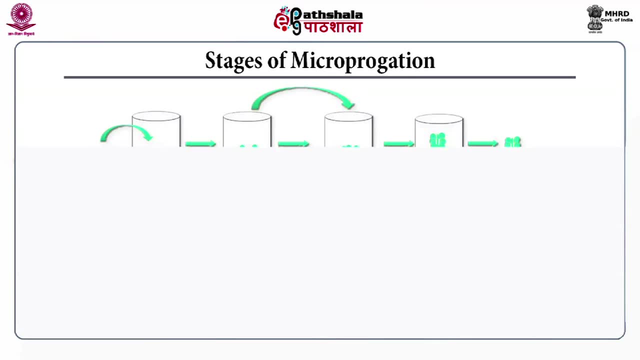 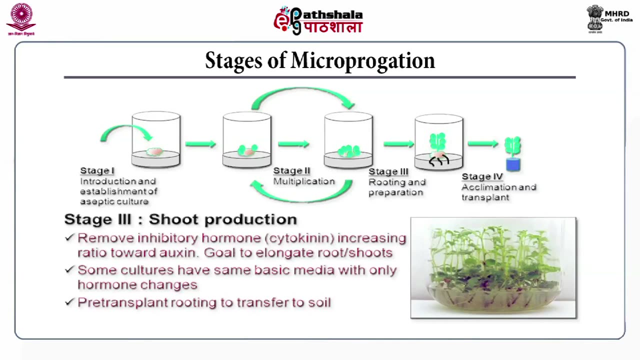 The micro propagation is rapid and has been adopted for commercialization of important plants such as banana, apple, pears, strawberry, cardamom and many, many, many ornamental plants. Here in this slide, The results of micro propagation are shown. 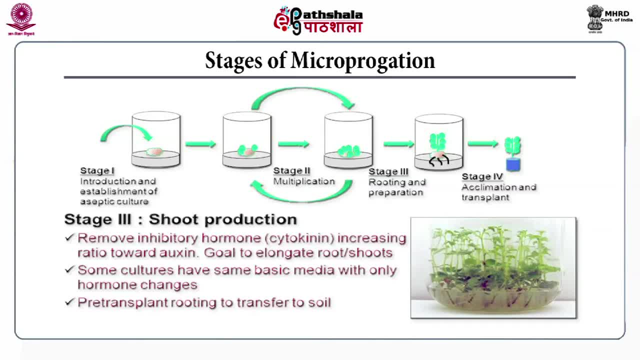 In the first stage there is introduction and establishment of aseptic culture. Then in second stage multiplication take place, and in third stage rooting and preparation is done, and in fourth stage acclimatization and transplanting take place. So this shows the different stages. 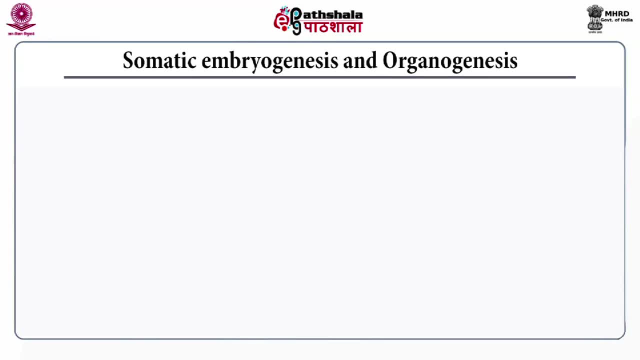 This is of micro propagation. Then third method is somatic embryogenesis and organogenesis. The development of somatic embryo from a single or multi cells is known as somatic embryogenesis. Plant propagation through somatic embryogenesis helps to obtain a large number of plants, irrespective 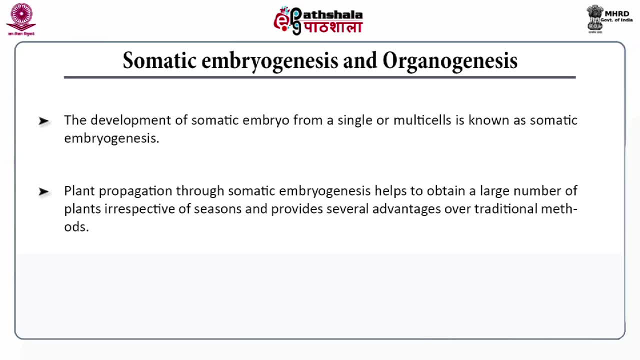 of seasons and provides several advantages over traditional methods. The main advantage of somatic embryogenesis is the production of numerous plantlets from a single cell, which provides an option for their screening and evaluation. The de novo organ synthesis, such as buds, roots and shoots from culture tissue is called 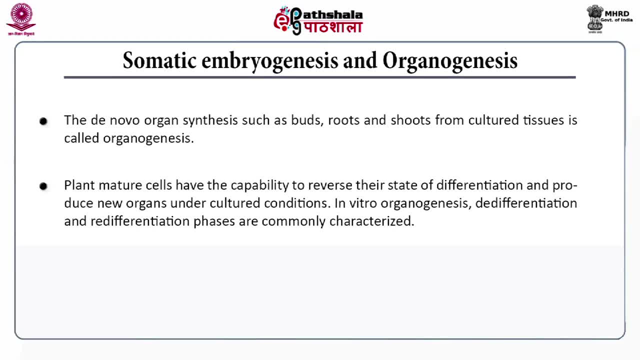 as organogenesis. Plant mature cells have the capability to realize and produce organogenesis, but not best reverse their stage of differentiation and produce new organs under cultured condition. In vitro organogenesis, de-differentiation and re-differentiation phases are commonly characterized. The balance of exogenous auxin and cytokinin in the medium is essential for 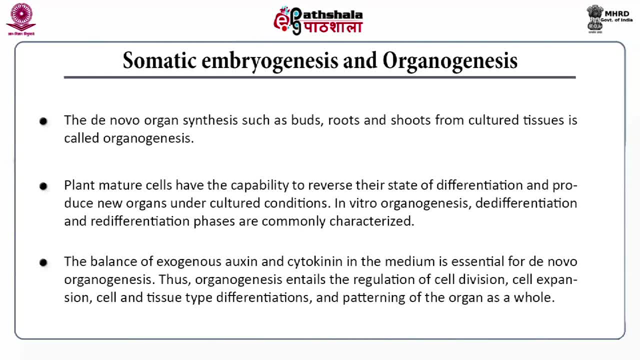 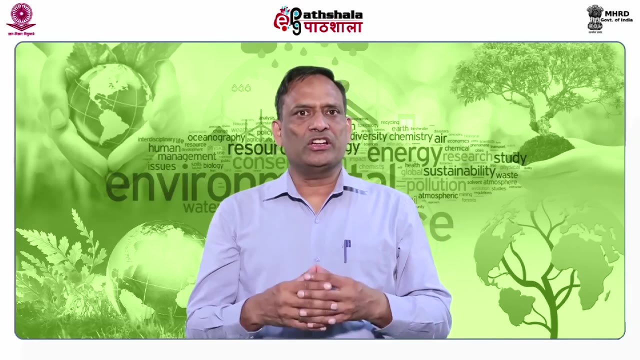 de novo organogenesis. Thus, organogenesis entails the regulation of cell division, cell expansion, cell and tissue type differentiation and patterning of the organ as a whole. Now the fourth technique under plant tissue culture. under tissue culture techniques is animal tissue culture, Two principal methods. 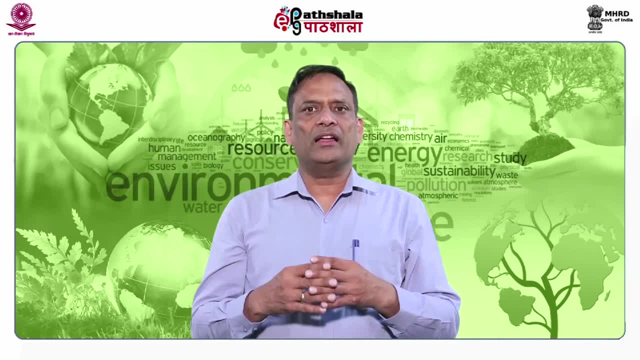 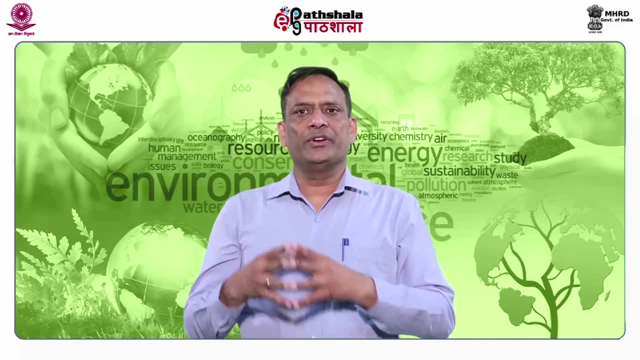 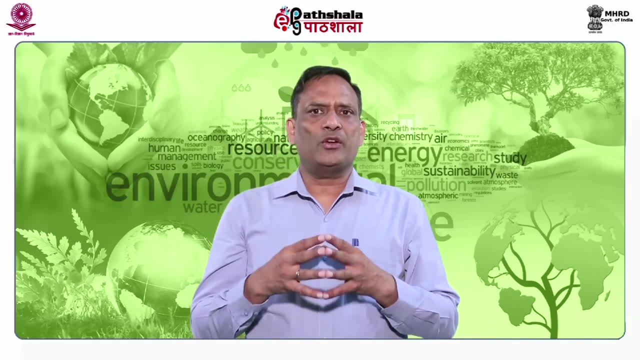 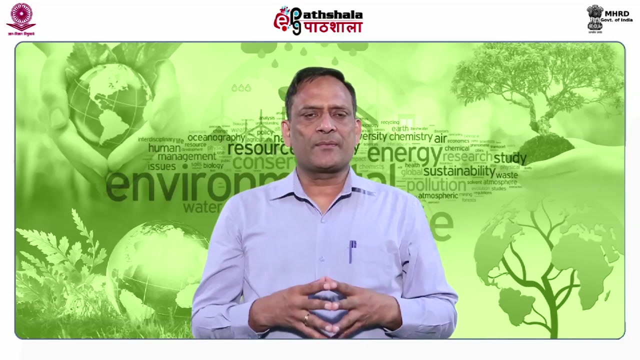 for conserving animal germ plasm. in vitro organogenesis Are as frozen semen and embryos. Both methods require the maintenance of female animals for either insemination or implantation. Embryos have an advantage over semen because they provide the complete genotype In some domestic species. embryos for transfer or 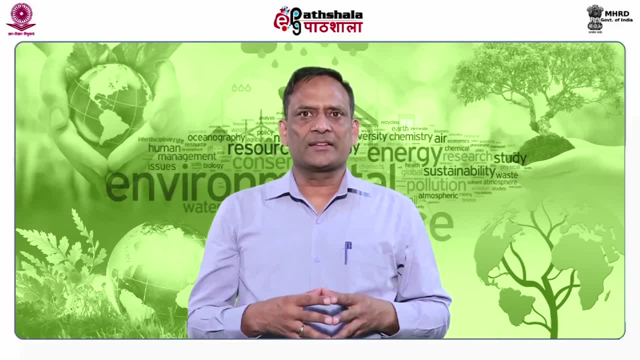 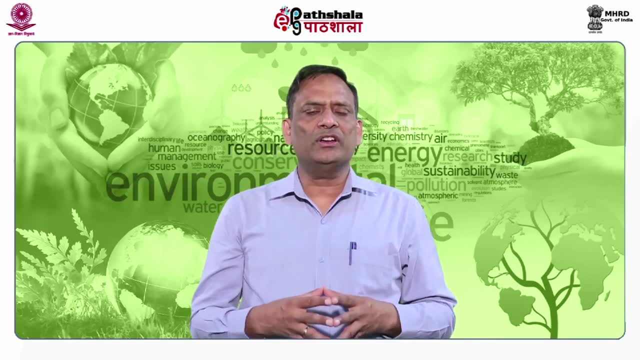 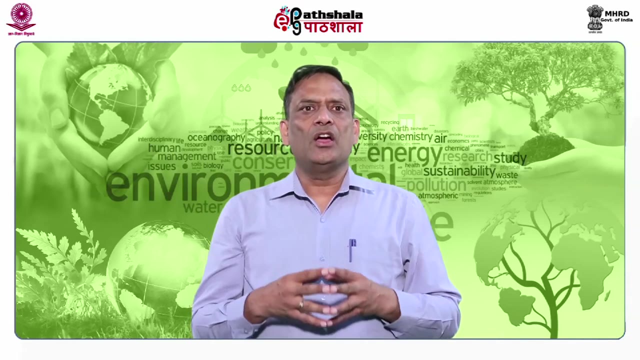 cryopreservation are collected from animals that have received hormonal treatment to induce an excess of eggs for insemination. The resulting embryos are evaluated for their potential to produce a pregnancy or to withstand freezing. Embryos from cattle, sheep, goats and horses have all been frozen in liquid nitrogen thawed. 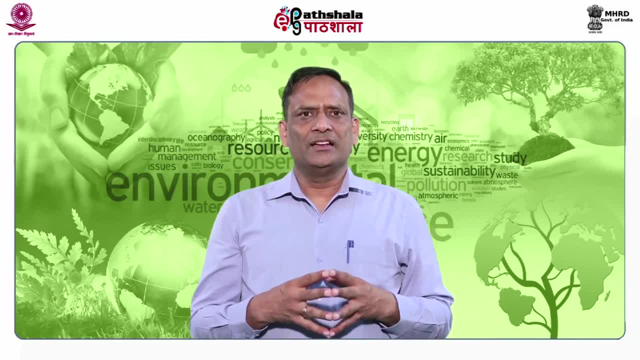 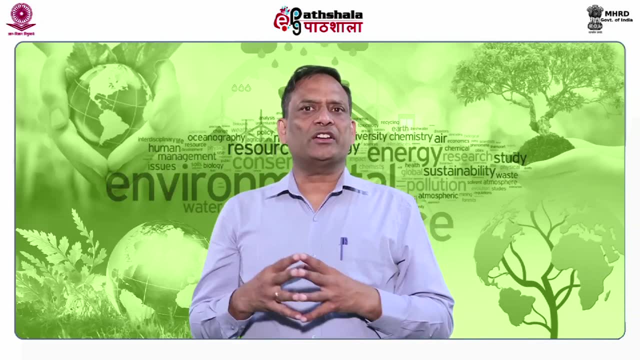 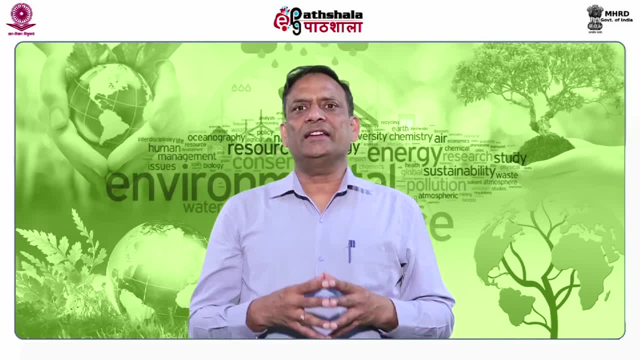 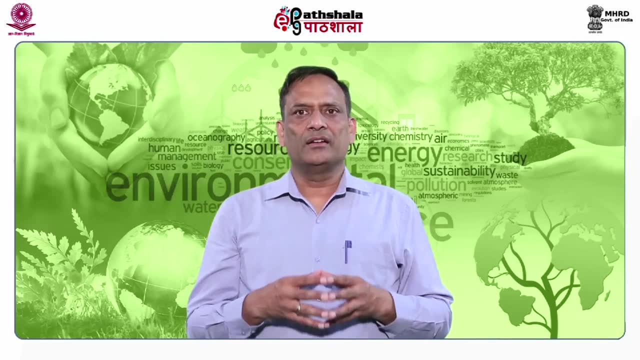 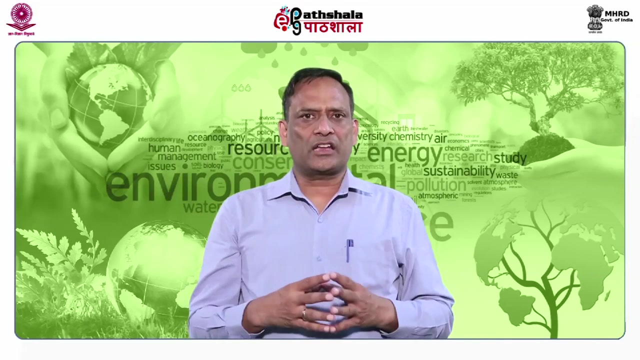 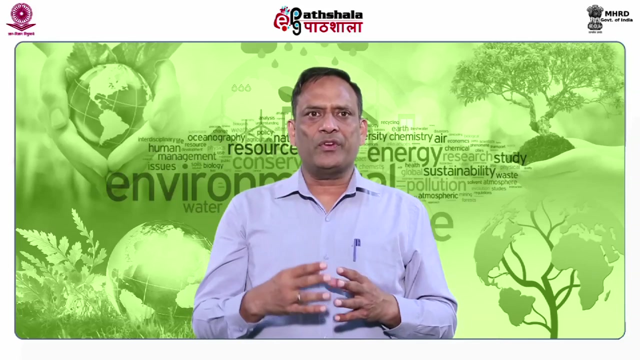 for long term storage of plant genetic material. Cryopreservation is extremely helpful method to conserve rare, endangered and threatened species. There are two types of cryopreservation protocols that basically differ in their physical mechanisms. First is classical cryopreservation procedures, in which cooling is preferred in the presence. 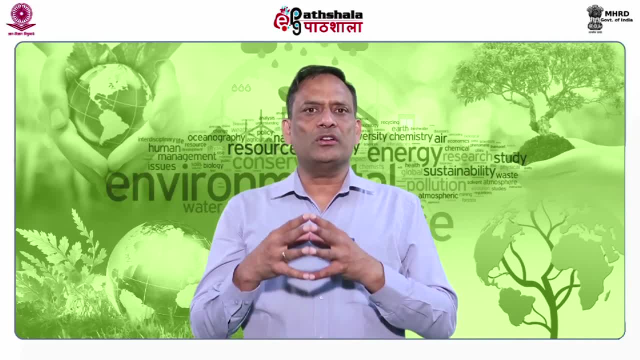 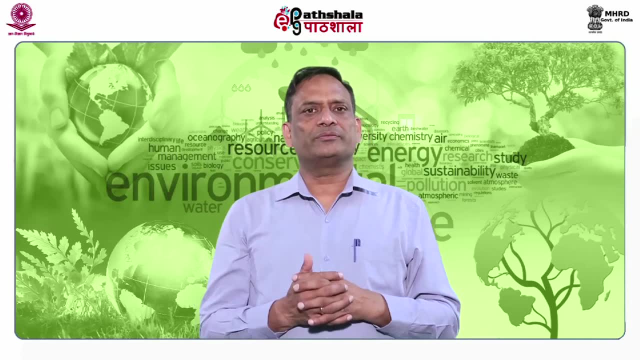 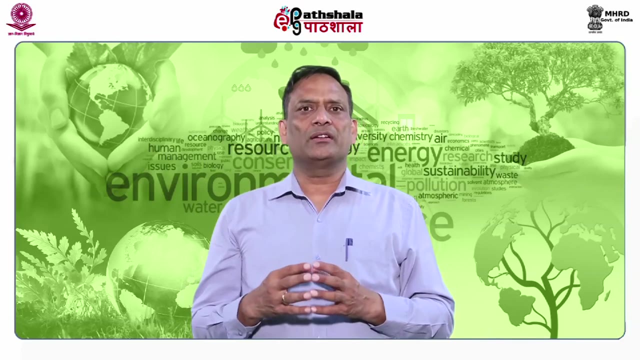 of ice and in the procedures based on vitrification, in which cooling normally takes place without ice formation. Classical freezing method includes the successive steps, such as pregrowth of sample, cryoprotection, slow cooling at 0.5 to somewhere 2 degree Celsius per minute to a determined 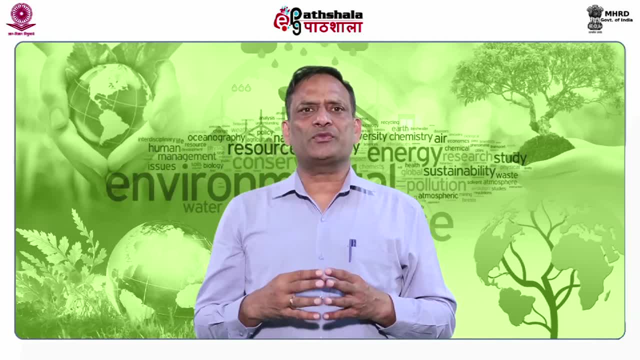 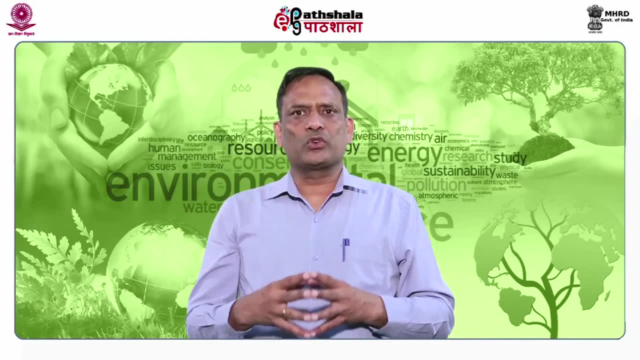 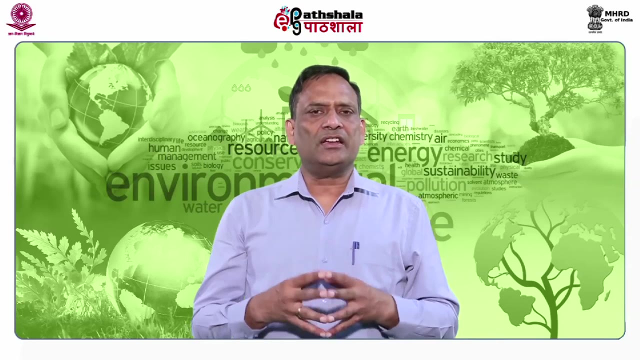 pre-freezing temperature, usually in the range of minus 40 degree Celsius, rapid immersion of samples in liquid nitrogen storage, rapid thawing and recovery. It needs technical skill as it has several steps: 1. Cryopreservation, 2. Cryopreservation, 3. Cryopreservation, 4. Cryopreservation, 5. Cryopreservation. 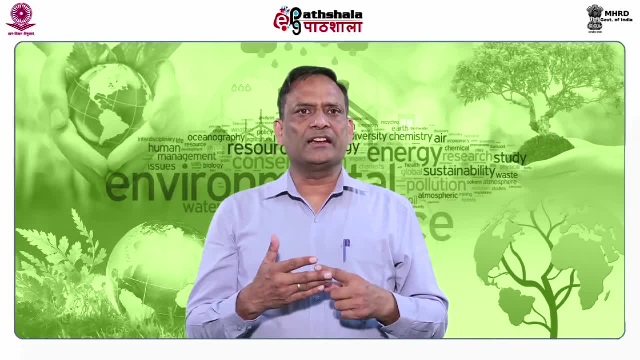 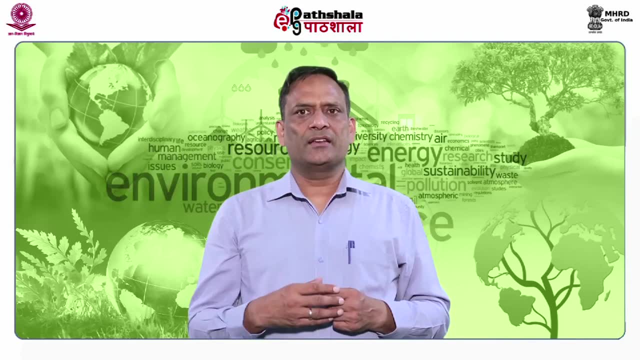 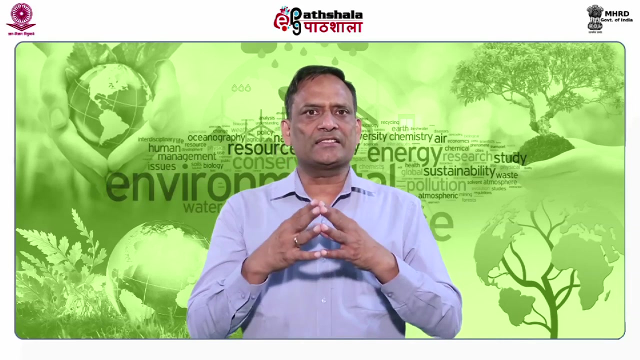 6. Crypemutação, Such as freezing, storage, thawing, reculture of living plant cells during cryopreservation against cryogenic injuries. Maintenance of cryogenic cultures in liquid nitrogen at minus 196 degree Celsius or in the vapor phase in liquid nitrogen at minus 135 degree Celsius is in such a way that the 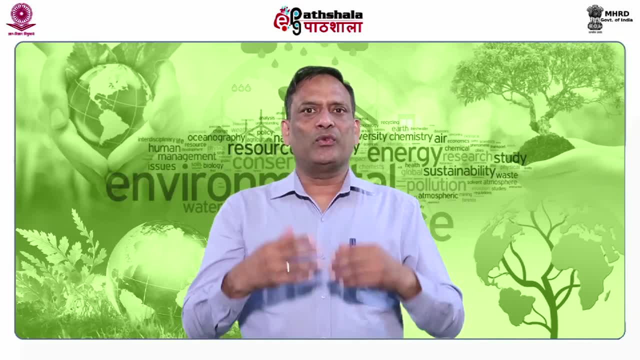 viability of stored tissues is retained, So it is not stealing An eating. standing outside the rotating chamber is torn fromMore pot than anything required, and so it has its own safety and fellow, so it is managed by it several times within the body of any living living being. Research in this German study has illustrated that. lay onto. 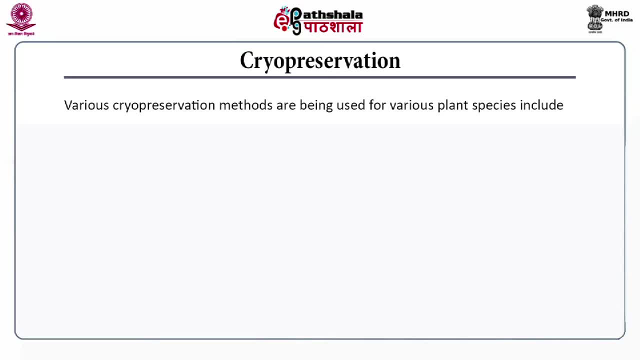 following rewarming. Various cryogenic methods are being used for various plant species, and these methods include vitrification, encapsulation, dehydration and encapsulation vitrification: Basically, vitrification comprises treatment of samples with cryoprotective substances, followed by dehydration with highly concentrated plant vitrification solutions. rapid cooling. 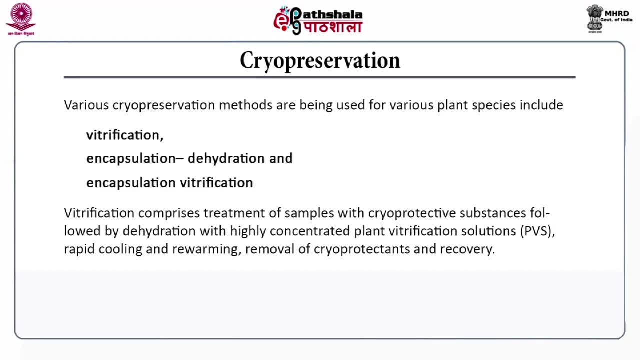 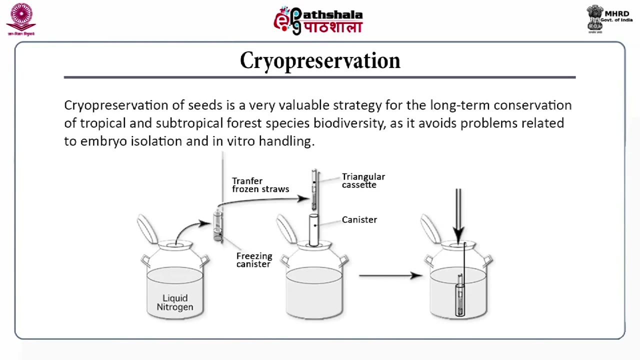 and rewarming, and removal of cryoprotectants and recovery. Cryopreservation using the encapsulation dehydration procedure has been very effective for freezing different plant species from temperate and tropical. Cryopreservation of seeds is a very valuable strategy for the long term conservation of 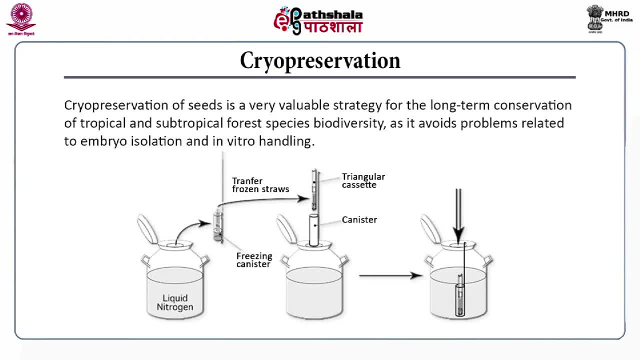 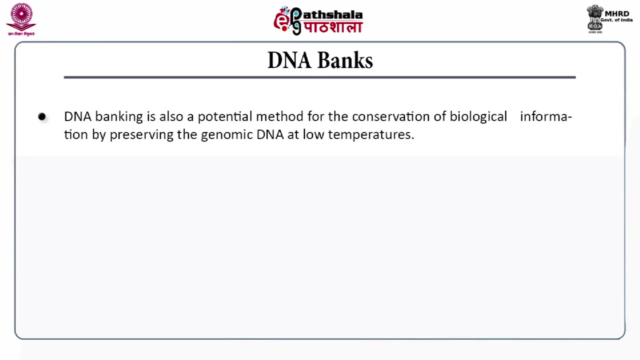 tropical and subtropical forest species. biodiversity, as it avoids problems related to embryo isolation and in vitro handling. In this picture you will see that there is a tank of cryogenic liquid nitrogen and how the material is preserved in the cryogenic liquid nitrogen tank. Then another method is DNA Banking. DNA Banking is also a potential method for the conservation 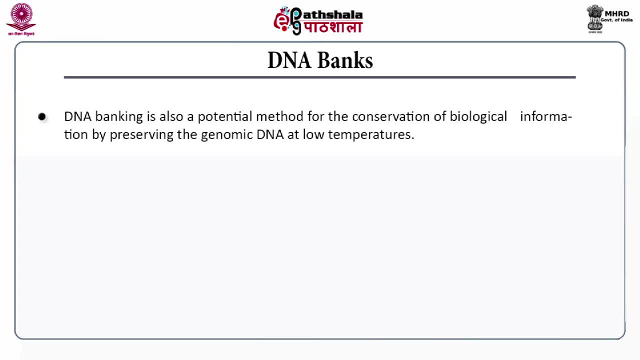 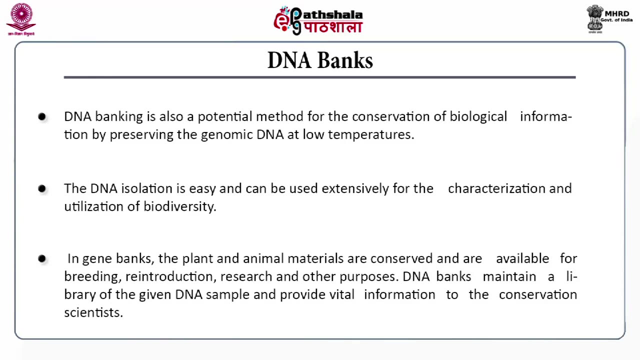 of biological information by preserving the genomic DNA at low temperatures. The DNA Banking is the best method to preserve the住宅match DNA at lower temperatures. A DNA isolation is easy and can be used extensively for the characterization and utilization of biodiversity. In gene banks, the plant and animal materials are conserved and are available for breeding. 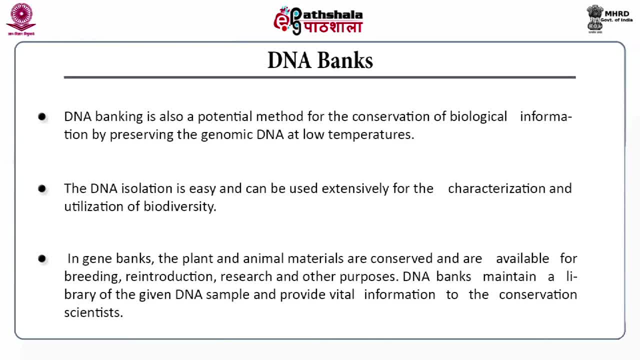 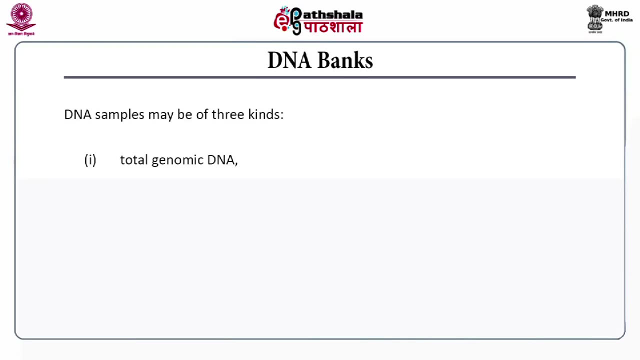 reintroduction, research and other purposes. DNA banks maintain a library of the given DNA sample and provide vital information to the conservation scientists DNA samples are. DNA samples may be of three kinds: total genomic DNA, DNA libraries and individual cloned DNA fragments. The maximum possible genetic diversity of the particular gene genetic stock can be. 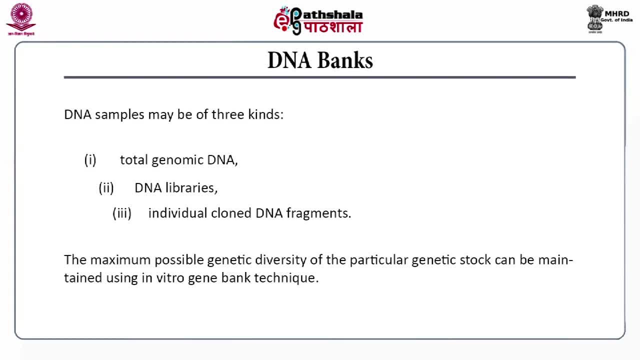 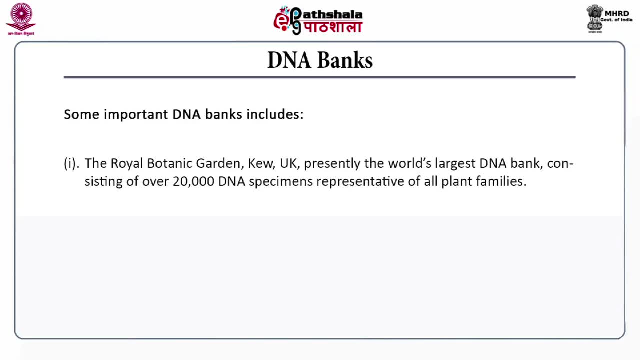 maintained using in vitro gene bank technique. Some important gene banks all over the world are include: the Royal Botanical Garden Q, UK, presently the world's largest DNA bank, consisting of over 20,000 DNA species representative of all plant families. The US Missouri Botanical Garden has collection of more than 20,000 plant tissue samples and. 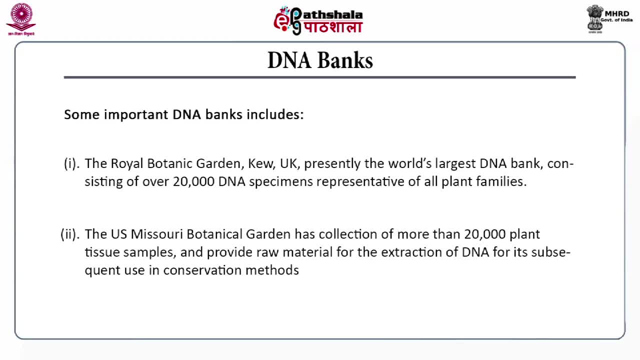 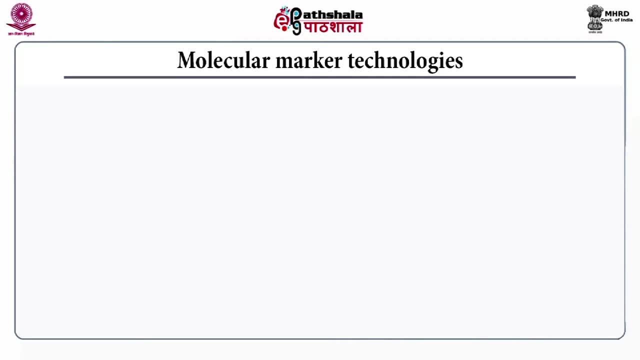 provide raw material for the extraction of DNA for its subsequent use in conservation research. Now second approach is use of molecular marker technologies for biodiversity conservation. Molecular marker technologies are discussed here include biochemical markers. Different variants of the same enzyme having identical or similar functions are known as isozymes. 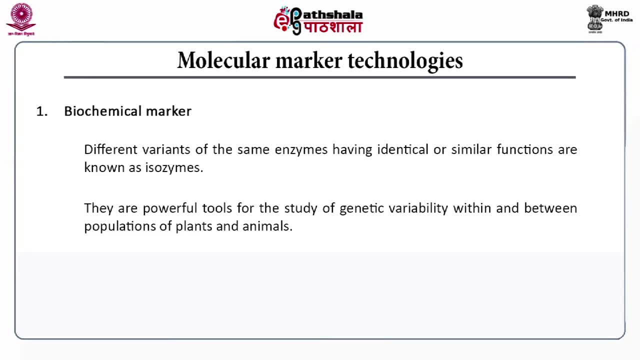 They are powerful tools for the study of genetic variability, Variability within and between populations of plants and animals. They are useful when several taxa accessions and individuals are to be compared, to identify clones and to examine the clonal structure of various plant population. Then we have phytochemical markers: The discovery 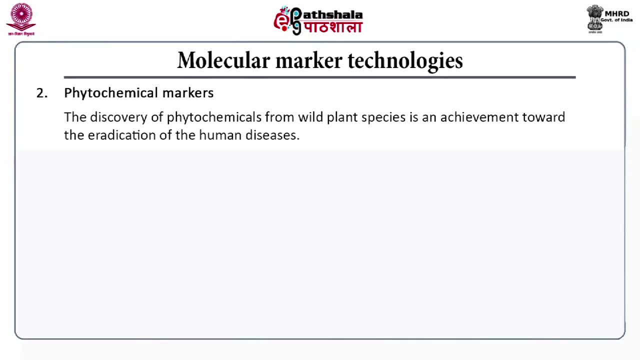 of phytochemicals from wild plants and animals. The discovery of phytochemicals from wild plants and animal species is a great achievement toward the eradication of human diseases. With the advancement of modern techniques such as mask spectrometry, NMR, that is, nuclear. 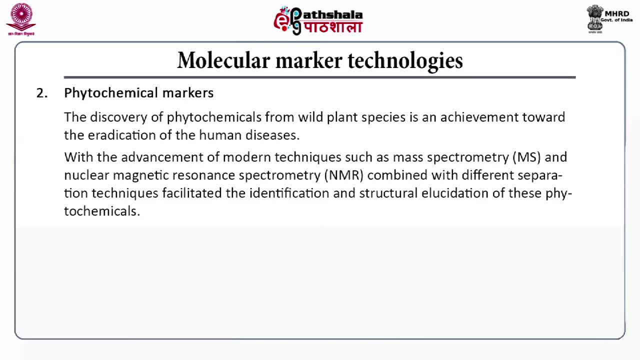 magnetic resonance spectrometry, combined with the different separation techniques, facilitated the identification and structural elucidation of these pharmaceuticals. These phytochemical analyses are valuable tools for manovers and functional healings. Since ancient times, theydasung andspecoloin пепеломые Ans lançались дляо 근�heitscat. dla нас necesit��는. 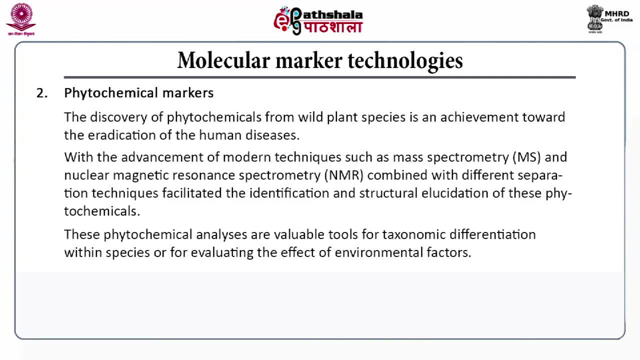 stem cell attache Officially commented in the requije of the patents for thiscemos isactive. that says thatсе케을 tools for taxonomic differentiation within species or for evaluating the effect of environmental factors. Variation in biosynthesis of these metabolites could be a result from both genetic and environmental. 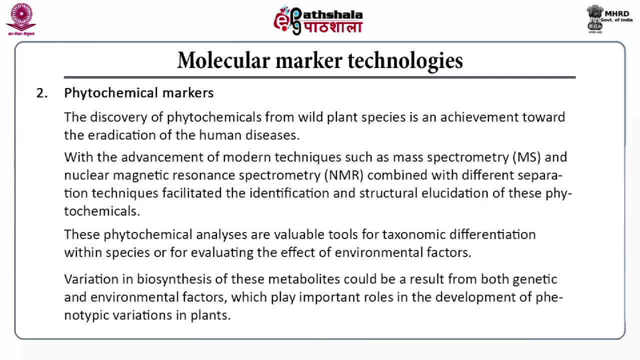 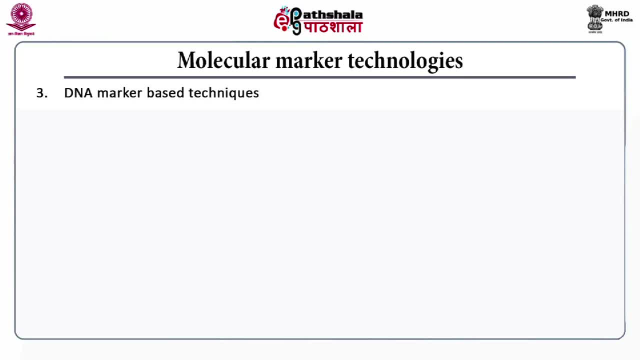 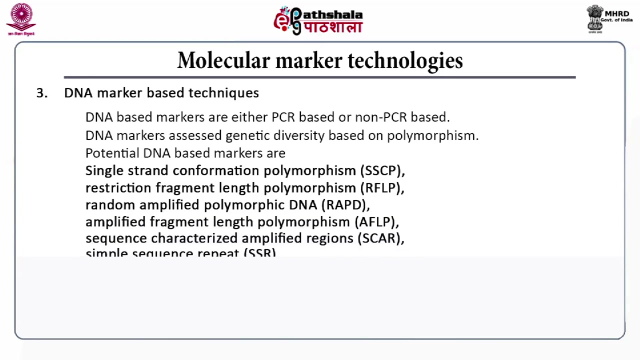 factors which play important roles in the development of phenotypic variations in plants. Then DNA marker. DNA marker based techniques. DNA based markers are either PCR based or non-PCR based. DNA markers assessed genetic diversity based on polymorphism Potential. DNA based markers are single strand confirmation polymorphism. SSCP restriction. 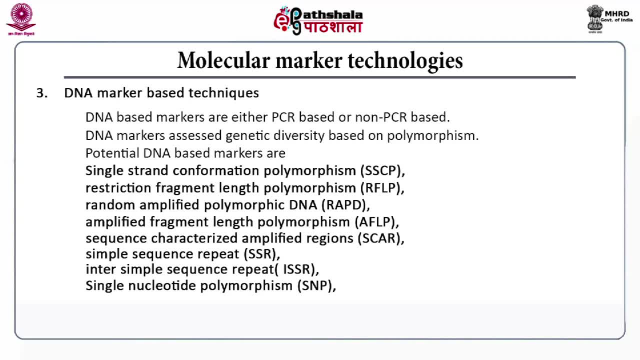 fragment length polymorphism, that is RFLP System. amplified polymorphic DNA, that is RAPD. Then amplified fragment length polymorphism, that is AFLP. Sequence characterized amplified regions: SCAR. Then simple sequence: repeat SSR. Inter simple sequence: repeat ISSR. 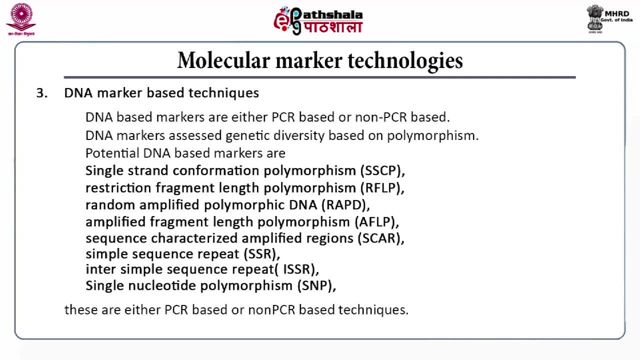 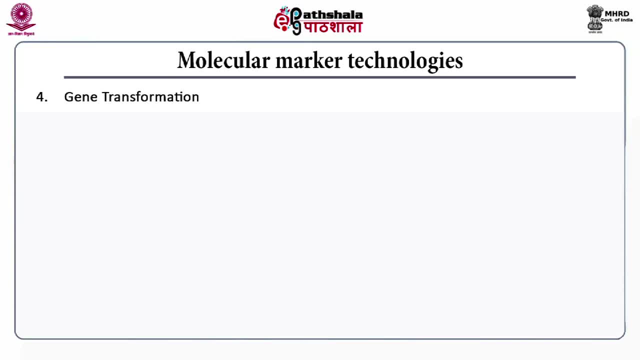 Single nucleotide polymorphism, that is, SNP. These are either PCR based or non-PCR based, So these all techniques can be used in biodiversity conservation in one or the other way. Then gene transformation. Gene transformation is a powerful tool for enhancing the productivity of novel secondary